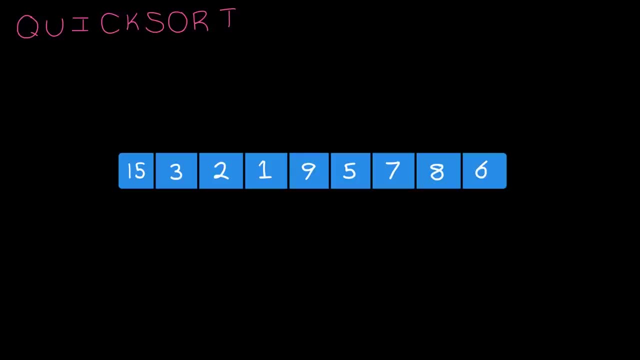 pick some element to be the pivot element. For now we'll just assume we're going to pick the pivot element randomly And what we do is we walk through the array and we swap elements around such that all elements less than the pivot come before all elements bigger than it And that 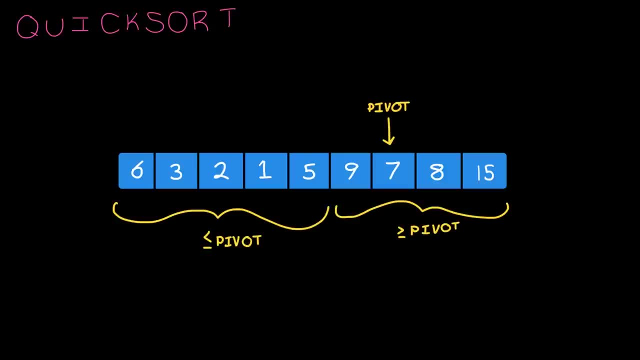 creates some sort of natural division in the array. And then we repeat this process and we apply this algorithm to the left portion and the right portion, And then we do that over and over again and eventually our array just becomes sorted. Let's drill into this in a little bit. 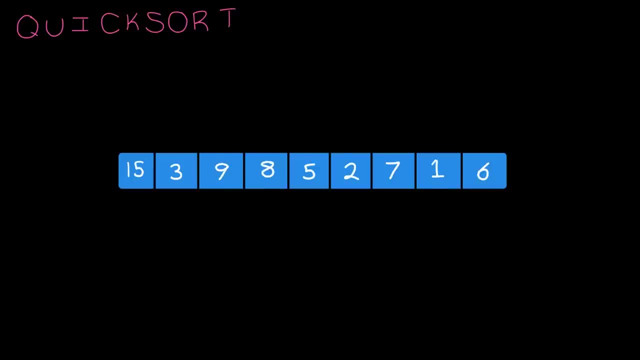 more detail now. We'll pick a pivot element randomly, let's say it's 7.. Then what we'll do is we'll walk through the array from both sides, left to right and right to left, and then we'll swap elements if they're out of order. Out of order meaning means that every element less than 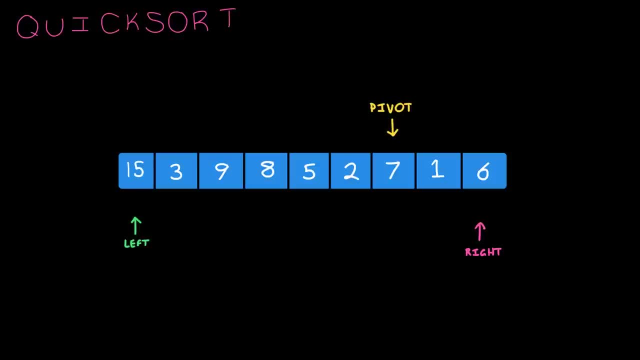 7 should be before every element greater than 7.. So first we have 6 and 15.. 6 is smaller than 7 and 15 is bigger than 7, so those should be swapped. Then we move this left pointer until. 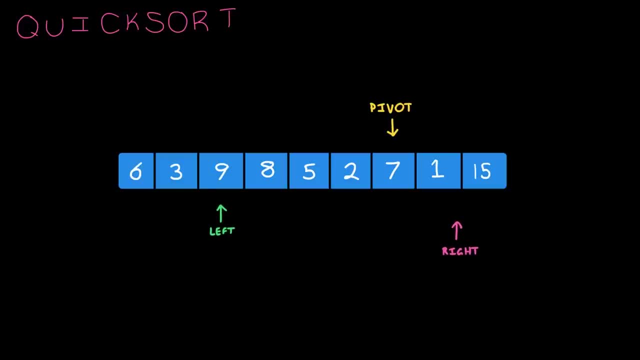 we find an element that should be on the other side and we do the same thing for the right. Okay, now 9 and 1, so those should be swapped as well. Take 1 over here, 9 over there. Okay, now again, move the left pointer until we have an element. 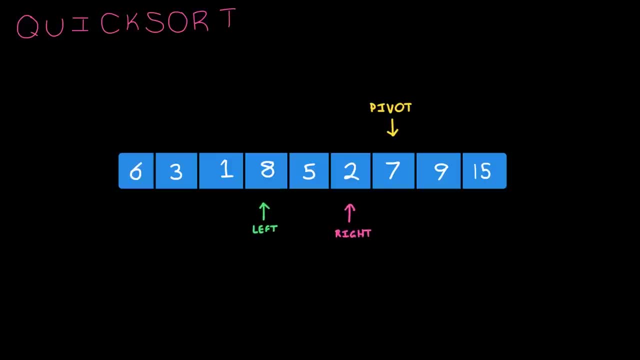 that should be swapped. Move the right pointer. Okay, 2 and 8, so those should be swapped. Okay, now we have an arrangement such that everything's smaller than the pivot is on one side and everything bigger than the pivot is on the other side. 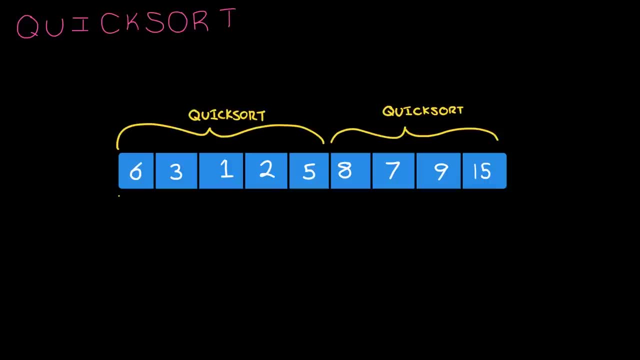 So now we just do quicksort on these two halves And on the left side we pick a pivot element randomly, let's say it's 3.. So then we walk through and move things smaller than 3 on one side and things bigger than 3 on the other side. So we have this left pointer and this right pointer. 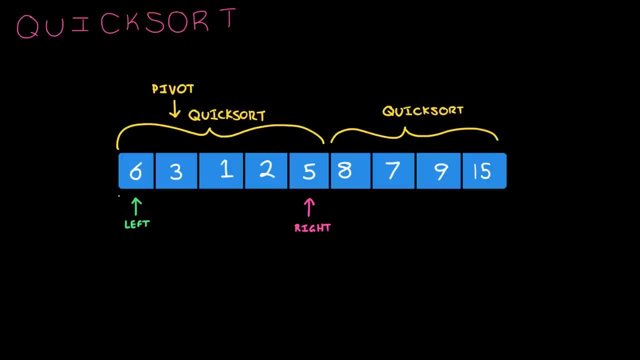 again. So we move the left pointer over until we have something that should be on the other side of 3 and move the right pointer over until we find elements to be swapped. So 2 is smaller than 3 and 6 is bigger than 3.. So we want to swap those elements Now. move the left pointer over. 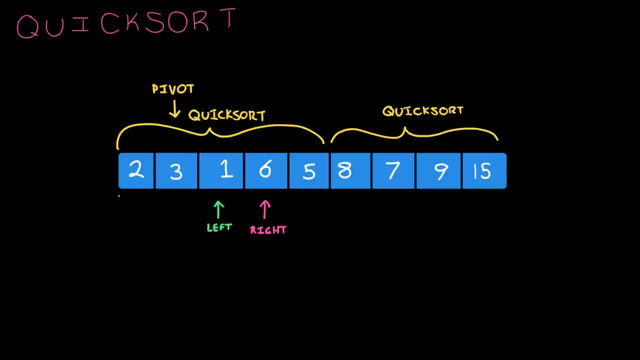 Until it has something that should be swapped, And we're good, actually. Okay, so now again we apply quicksort on each side. Okay so if we do quicksort on this very leftmost part now, we'll pick a pivot element randomly again. Let's suppose it's 2.. So then what we're? 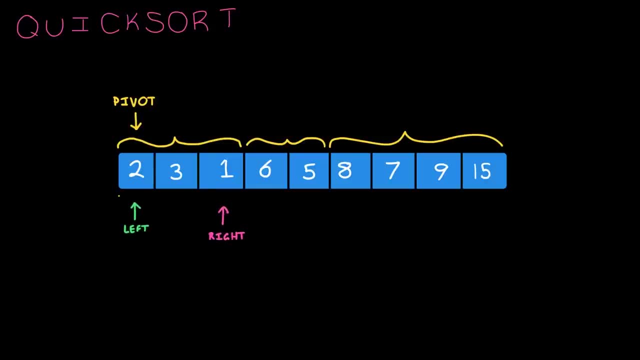 going to do is we're going to set the left pointer over here, the right pointer over here, Swap these elements around until we have elements that should be moved, So move this pointer over. So this left pointer will get moved over here. 3 should be on the right side and 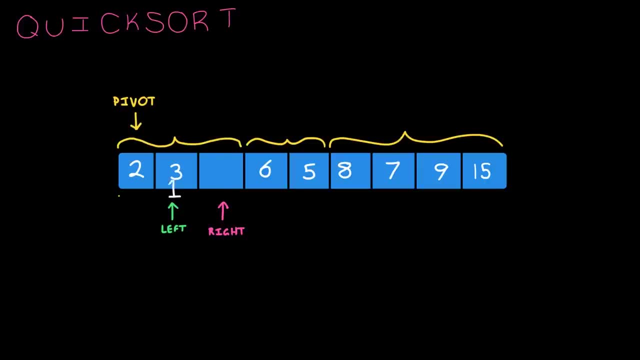 1 should be on the left side. So we're going to swap those elements And now we're actually done with this part. Then we want to apply quicksort to each of those parts. So, as you can see, this is getting progressively more and more sorted, And when you do this enough times, eventually we will wind up with a 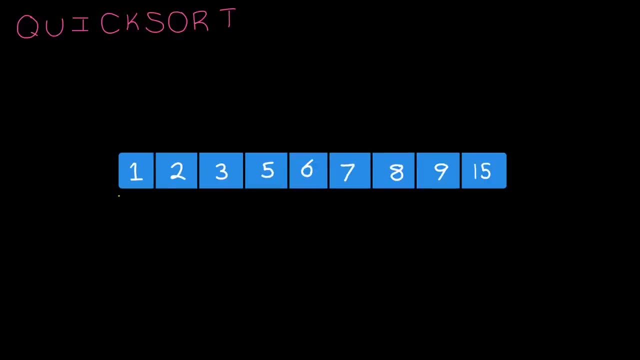 sorted array. So now the next question is: how efficient is this sorting algorithm? Well, in an ideal world, in quicksort we're dividing the array in half. each time We pick a great pivot- that really is roughly the median- And half the elements get pivoted to one side of the array. half of them get pivoted to the other. 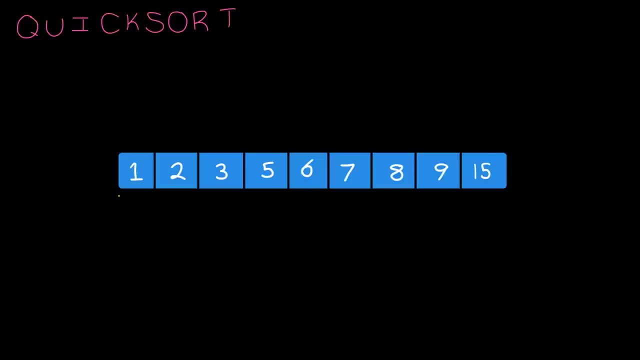 And then we just apply quicksort to each half. In that case we get an n log n runtime. One quick and dirty way of seeing why this is n log n in the good case is that each element gets quicksort called on it. 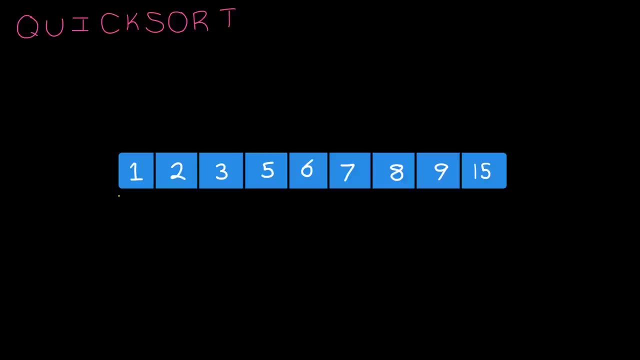 and if the other element is in common, then this is the best way to see why this is n log n In the good case is that each element gets quicksort called on it, gets quicksort called on it log n times And each one of those is one swap. So there's n elements. 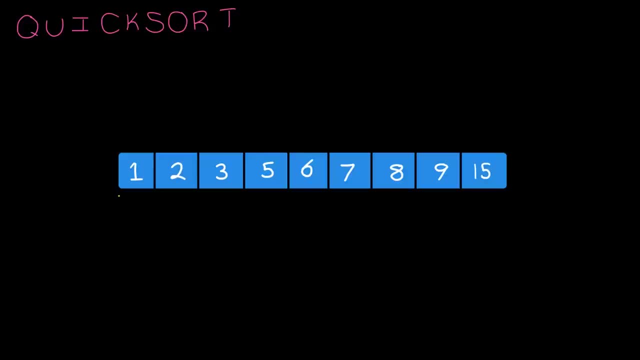 and they go through log n swaps, Then it'll take n log n time overall. However, in the bad case- let's imagine what happens here- We pick a really bad pivot. Like every time we pick the pivot element, it happens to be the very first element in the array or the very lowest element in that. 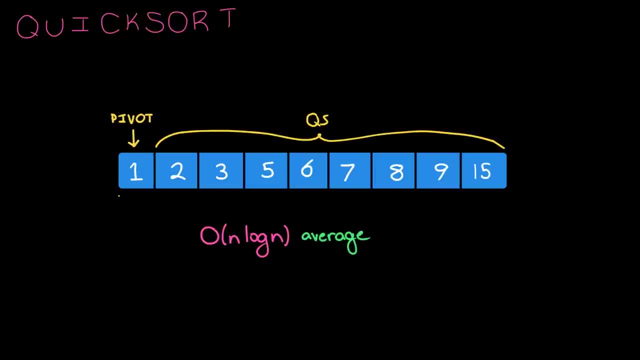 subarray. Then we actually have n squared calls to quicksort And therefore our runtime degenerates to o of n squared. But as long as we're smart about how we pick the pivot element, we can get a pretty efficient runtime And that's why we typically implement quicksort in the real world. 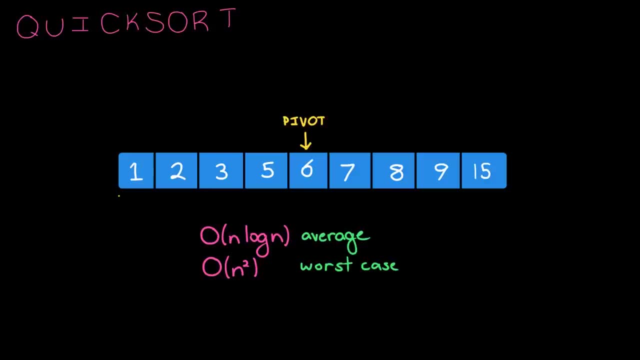 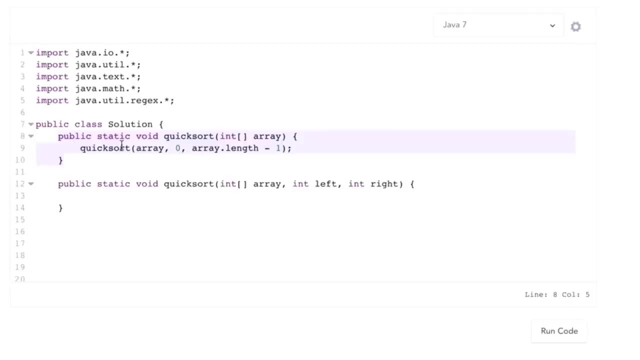 So now that you've seen how quicksort works at a high level, let's turn to the implementation. We'll implement quicksort recursively, So we're going to give ourselves this kind of overall method, initial method that we call. that goes n. 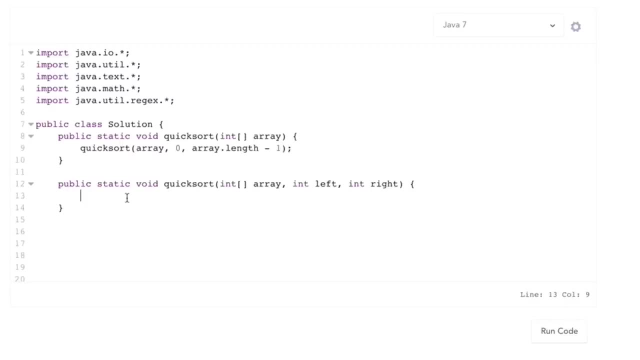 then calls the recursive method with the correct values. So first thing I want to do is I'm going to do a quick bounds check. So if left is, or if it's greater than or equal to right, then there's nothing to do, So just return. Okay, now I'm going to what I 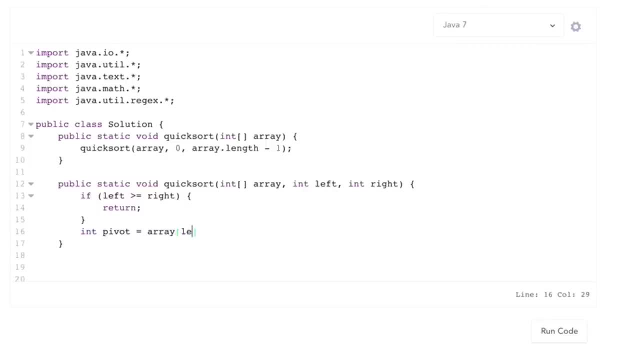 want to do is I'm going to pick a pivot element first. So I'm going to pick pivot to be right in the center there. but there's other ways you can do it, So pick it to be the center. Then I'm going to want to partition my array around this pivot, So call partition the left. 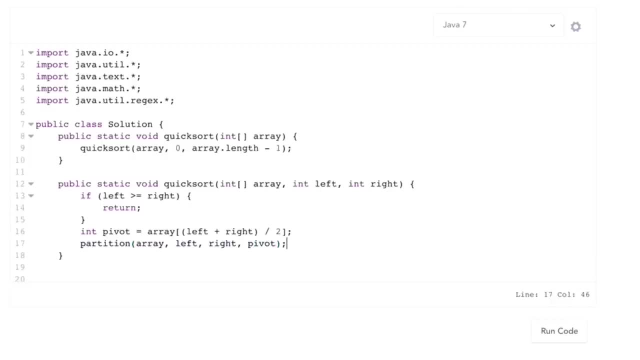 side, the right side, and this pivot value, And now partition is actually going to return the partition point. So return that dividing point between the left and the right side, And so I'm going to call that index And then, once I have that, I want to sort on the left and the right. 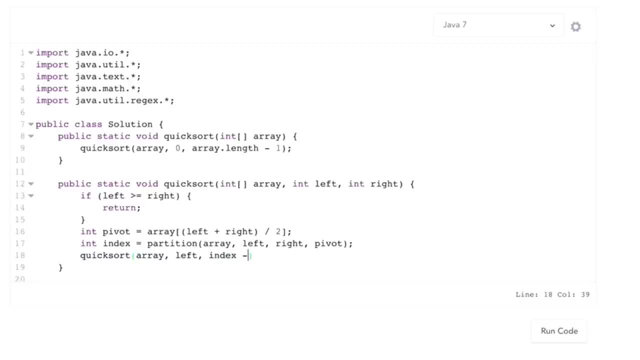 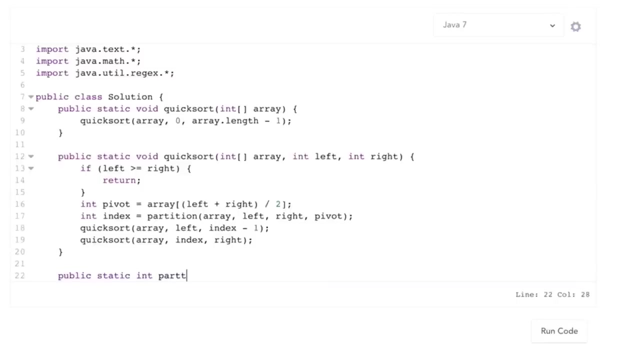 side. So call quick sort of left and the left side And then quick sort on the right side of that, And that's our basic framework. So now we just need to implement partition. Okay, so to implement partition now I need to take in a, I need to return an. 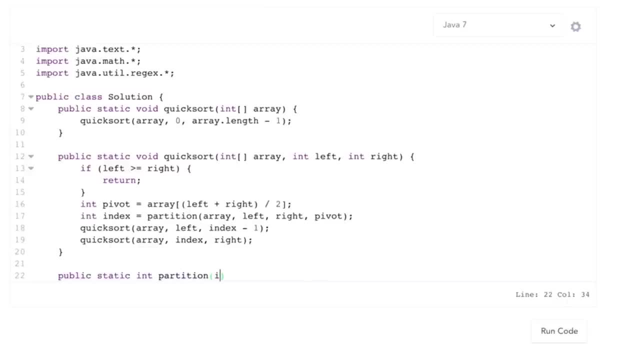 integer, which is going to be that partition dividing point, and it's going to take in the array, take in the left, take in, and there we go. So now I'm going to import that, So I'm going to, and there you go. So now I'm going to import that, So now I'm going to import that, So now I'm going to. 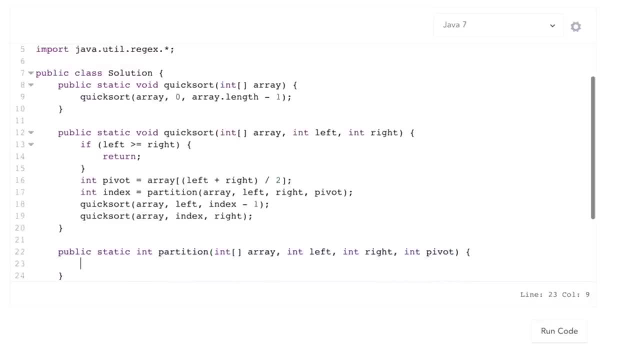 right side, and then this pivot value, And then what it's going to do is it's going to move, starting from the left side and the right side simultaneously. So move these pointers in towards each other. So, while left is less than or equal to, 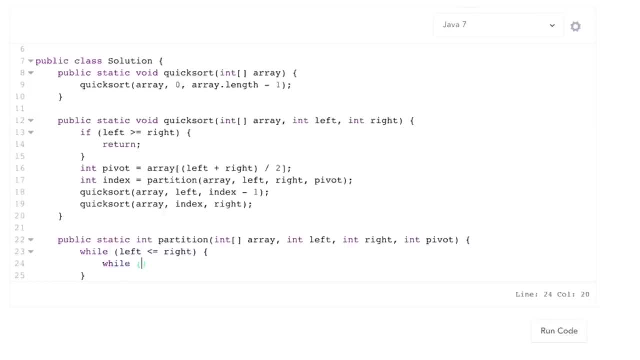 right. Now I want to move left until I find an element out of order. So the idea here is: look for an element on the left part that is bigger than the pivot, because then it should be on the right side and do the same thing on the right. 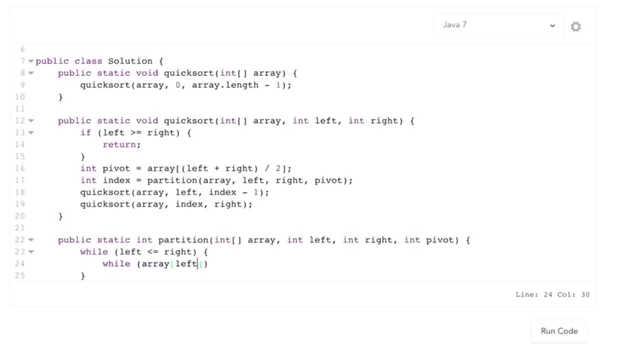 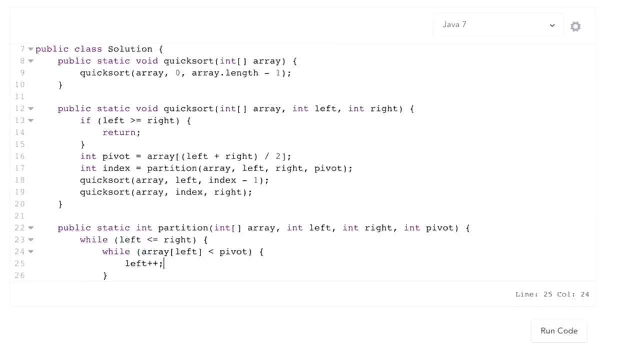 side. So while these elements are in the right place, so while array of left is less than the pivot, keep moving left. So this will break when I get an element that should be on the right side And then do the same thing on the right. 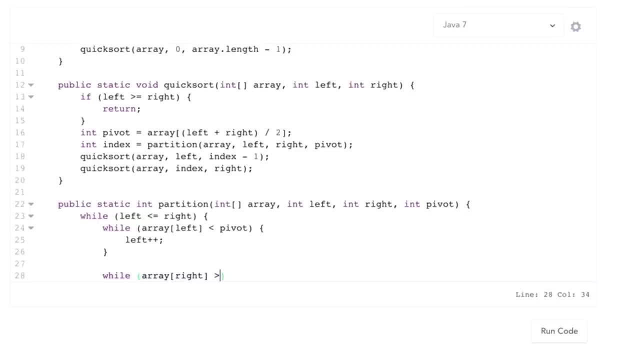 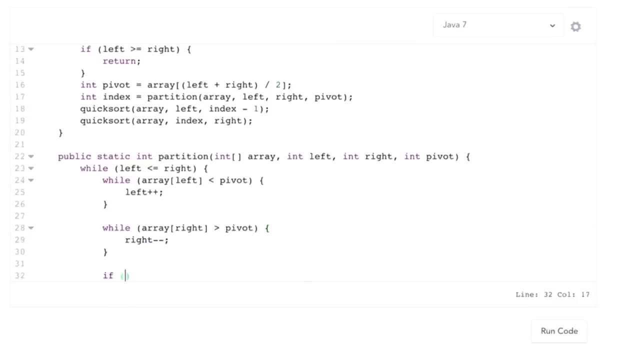 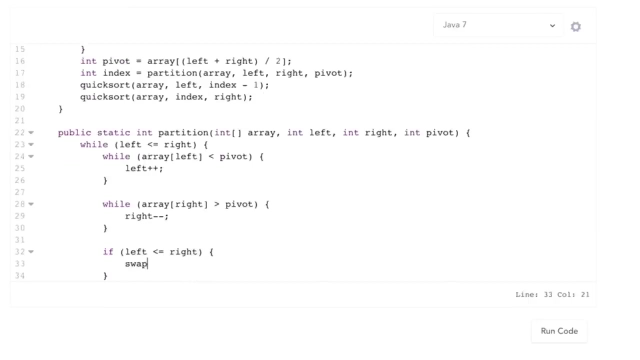 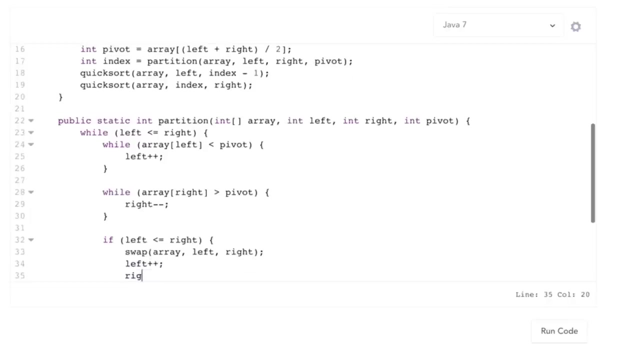 side. So while array of right is greater than the pivot, move that one inwards. Then if left is left less than right, since it's less than or equal to right, then swap those elements, So swap array, swap the elements of these two indexes and move left and right over. 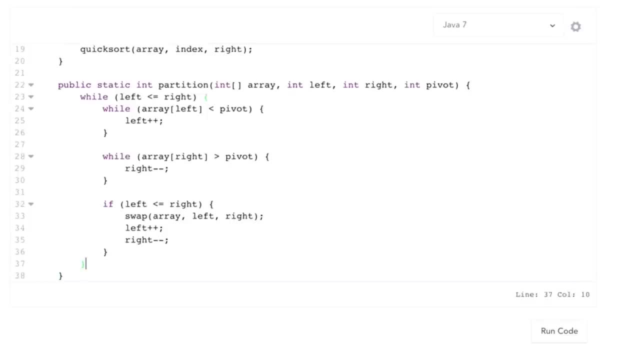 Now, when we get to the very end of this while loop, the elements will be in the right order or the elements will all be in the right order, So you'll have elements smaller than the pivot before all elements bigger than the pivot. Then we need to. 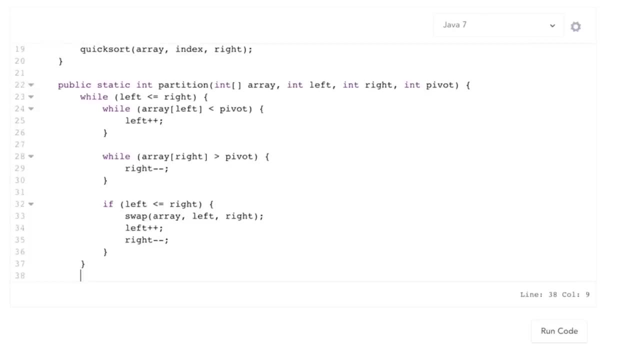 return the partition point. So we need to return that essentially dividing point between the left and the right side, And that is going to be where left is. That will give us the partition point. So that's how quicksort works. So let's walk through this again. So we call this: 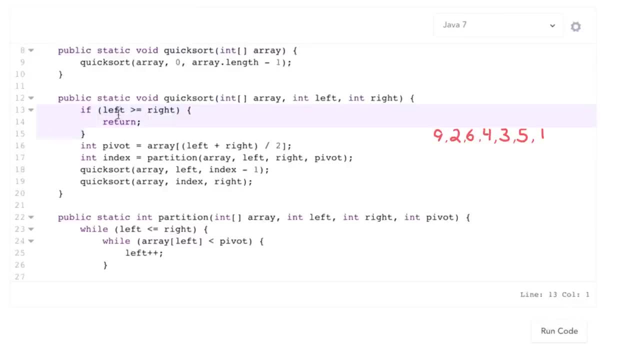 recursively The left and the right side are. if these indexes are out of order, then we just return. there's nothing to do. Then I pick the pivot, I partition these elements around the pivot and then I sort each side, And then let's look at. 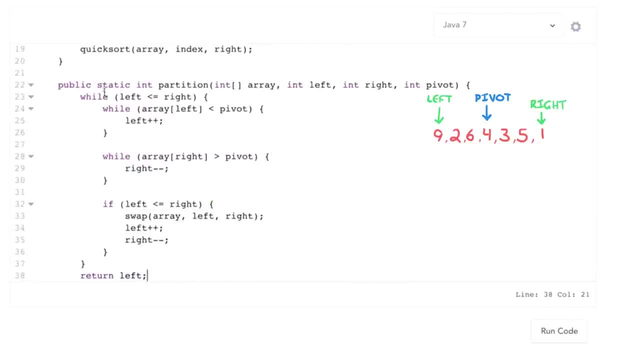 how partition works again. So I start from the left and right side, moving these pointers towards each other. I move the left pointer first until I get an element that is smaller, is bigger than the pivot, because that should be on the right side. Then I move the right pointer. 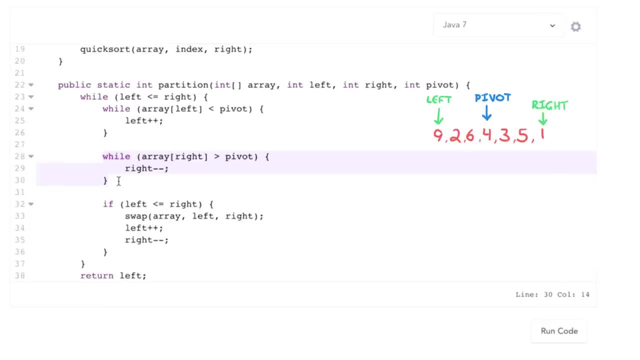 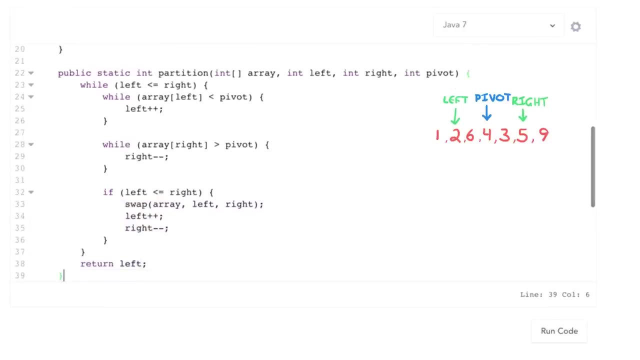 until I get an element that is smaller than the pivot, because that should be on the left side, And then I swap these values and move these indices. At the very end, left will be at that partition point. so I just return that Now, of course, in the 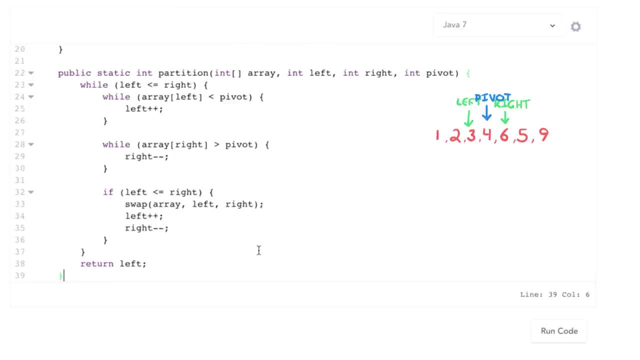 real world, we generally wouldn't implement a sorting algorithm from scratch, but it's still useful to understand exactly how they work. So now that you've seen the implementation, why don't you try applying a sorting algorithm to another problem? Good luck.